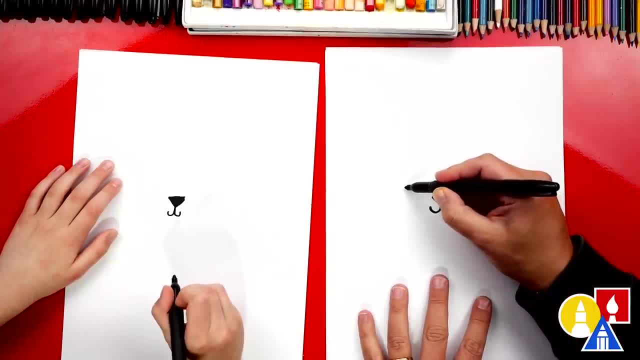 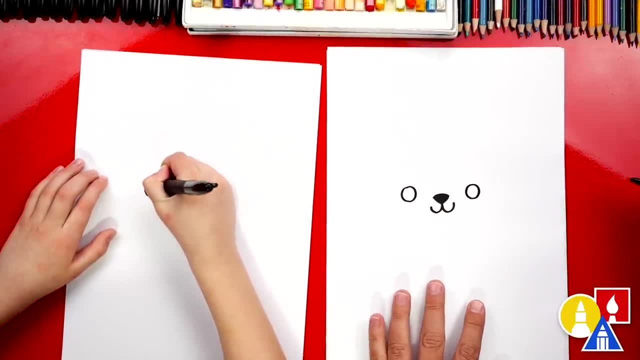 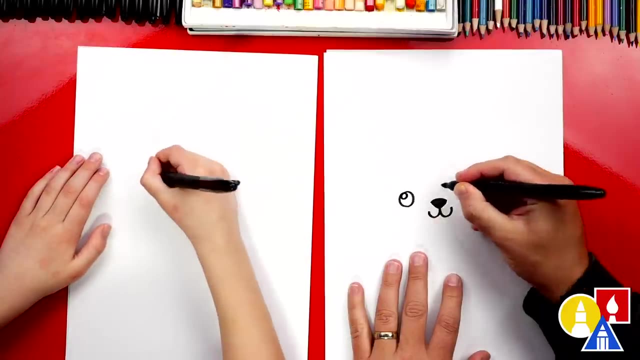 Then let's draw our panda's eyes. We're going to start over here and draw a circle about this size, And we're going to draw another circle the same size on the right. Yeah, Now let's draw a small circle or oval in the top left. 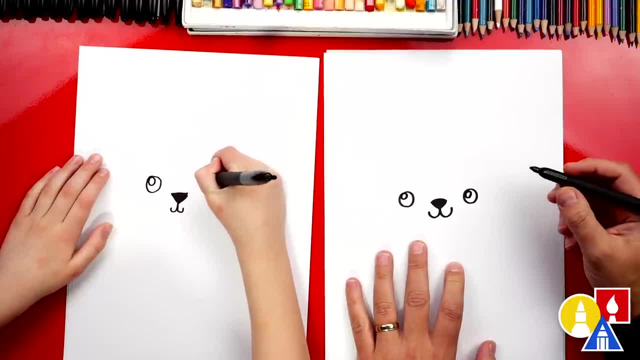 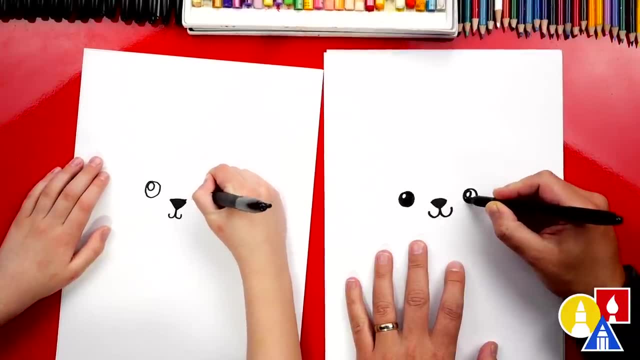 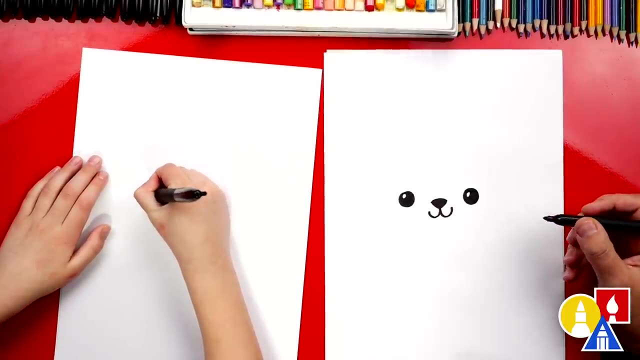 The highlight. make our panda's eyes look shiny and friendly. Yeah, leave the little circle white. Yes, we say that a lot, don't we Remember to pause the video when we fast forward or if we go too fast and you need extra time? 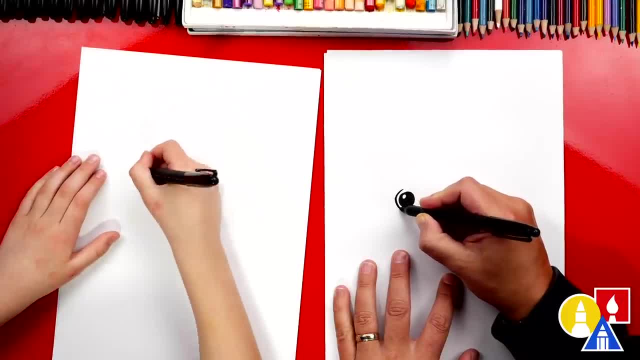 Now let's draw another circle around each eye. This is because we're going to draw spots around the eye. Make sure that I focus on the Tanzanianがとう's eyes, Since you love them. we're just going to use this, let it go. Just cut them out. Don't worry about the star pressed eye. Look for them, dude, You'd be fine with the star pressed eyes. So now let's draw a draw circle around each eye. This is because we're going to draw spots around each eye. 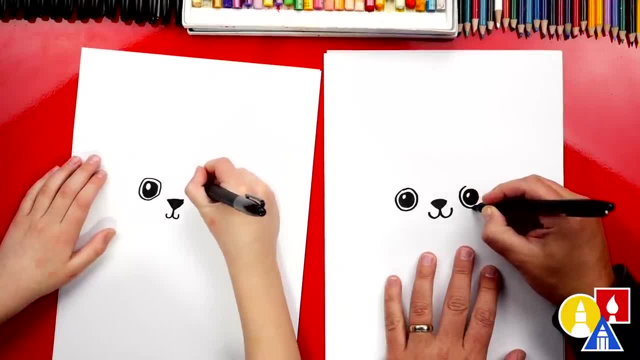 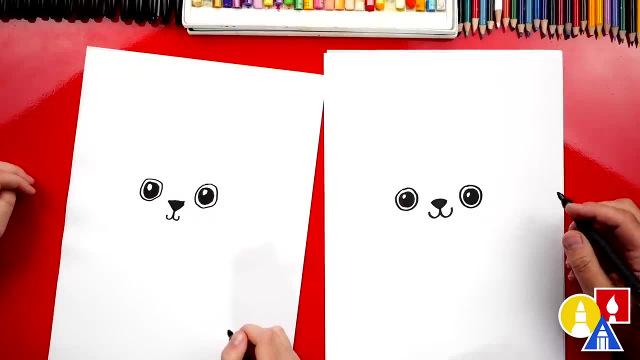 Now let's draw a draw circle around each eye. So our top》 this circle and top this circle and the top our pandas eyes. and we don't want to just color in the whole thing black. there we go. oh, it's already starting to well, not quite okay. now let's draw our 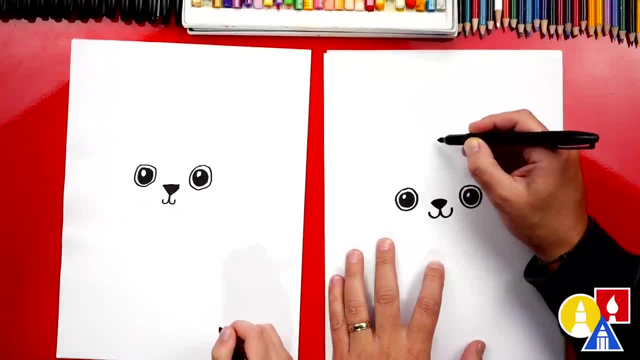 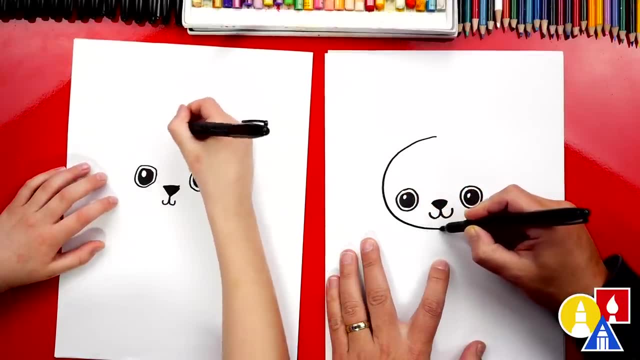 pandas head. we're gonna draw a big circle, but I'm gonna start. let's see, we'll start up here and draw a big circle that comes around. I'm gonna come close to the mouth down here at the bottom and then we're gonna come back up. 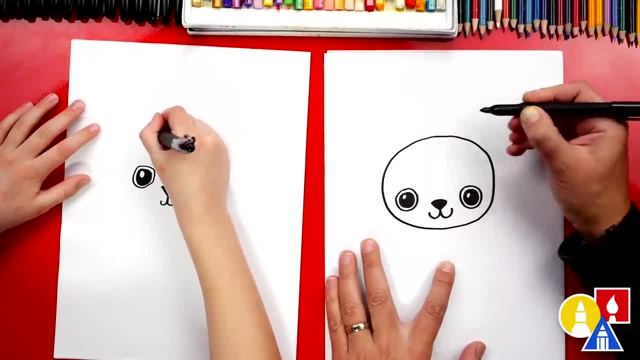 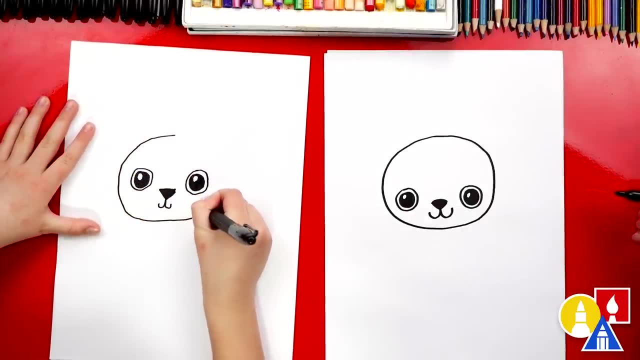 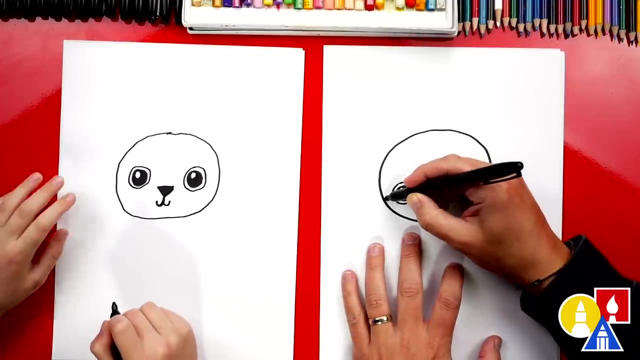 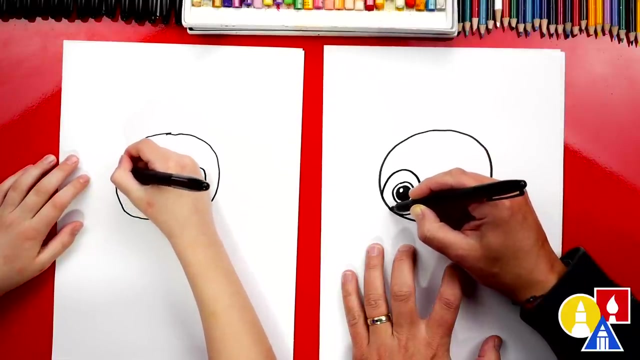 and connect to the top where we started. now we're ready to draw the spots around our pandas eyes. we're gonna draw an oval that comes around like this and I'm gonna touch the outside of his head or her head like that. yeah, if you have more, 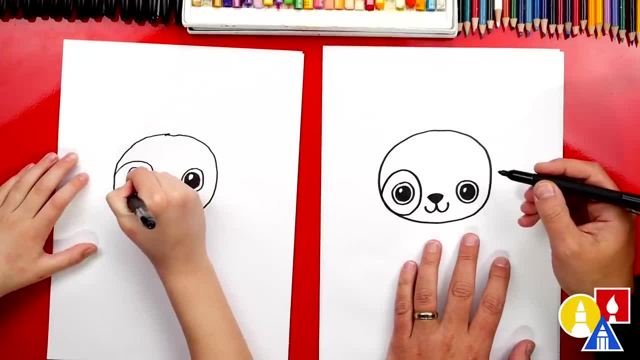 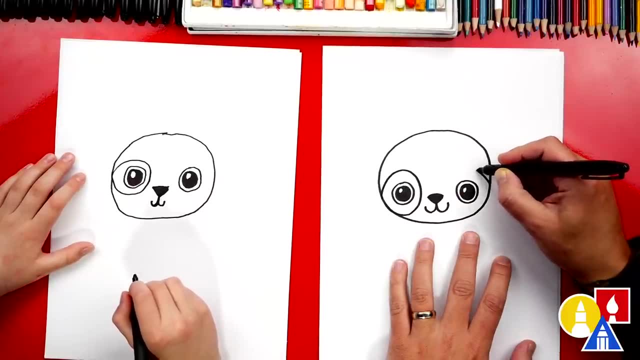 room. you could just draw the spot around. oh, I love the way that you did it. good job. now let's draw the same spot over here on the other side. I'm gonna try to make it look the same, but that's okay if it looks a little different and 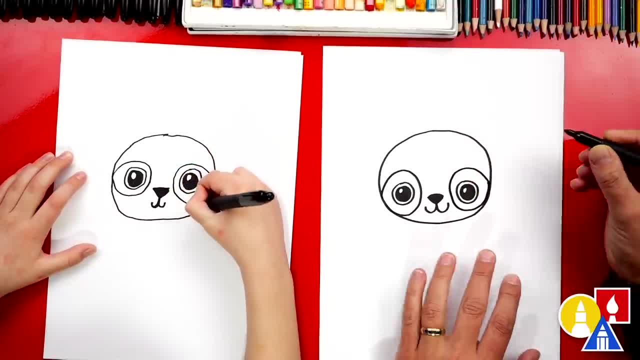 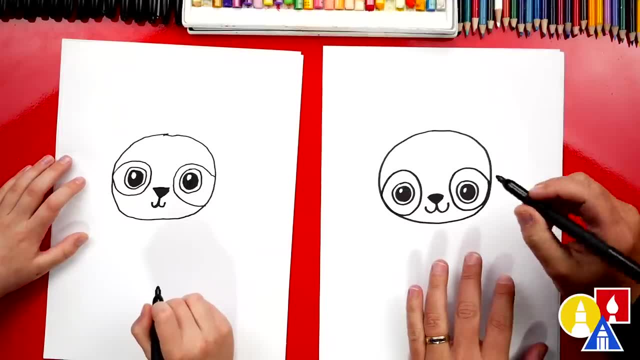 I love that our two drawings don't look exactly the same, because the most important thing is to have fun, yeah, and to practice, practice, remember to practice. all right, now let's draw our pandas ears. we're gonna draw an upside-down- you over here on the left. 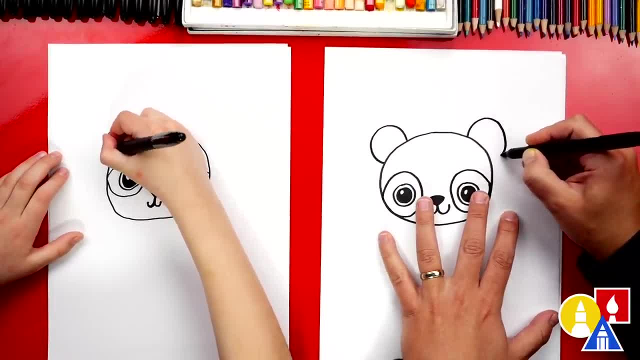 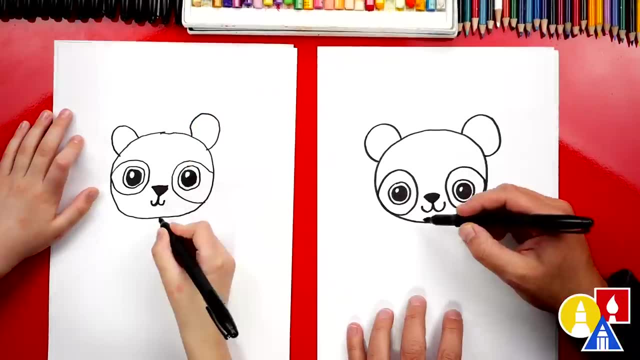 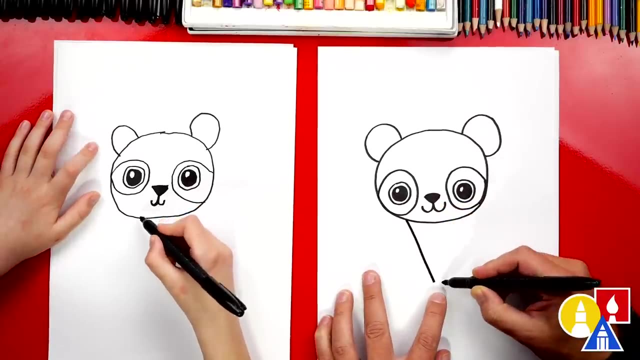 and also on the right. those might be a little too big for Panda ears. that's okay, I like the size that you're drawing. now we're gonna draw the paws, the front paws coming down, so let's start here and we're gonna draw a letter V. but look, I'm 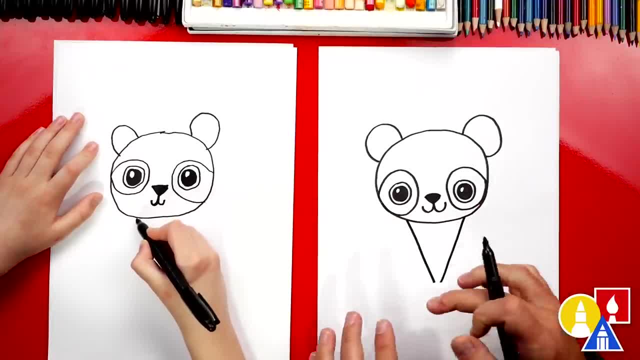 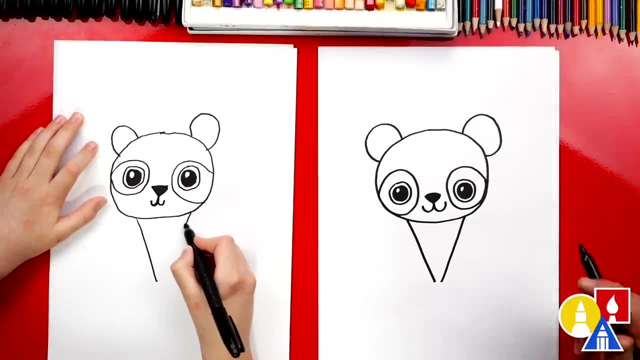 gonna leave a little gap at the bottom so you can draw two diagonal lines. you could also drop: oh yeah, just keep going, you're doing great there, you go, and then another diagonal line coming down and then a little more diagonal line over here, so I could draw a little bit of that working that. 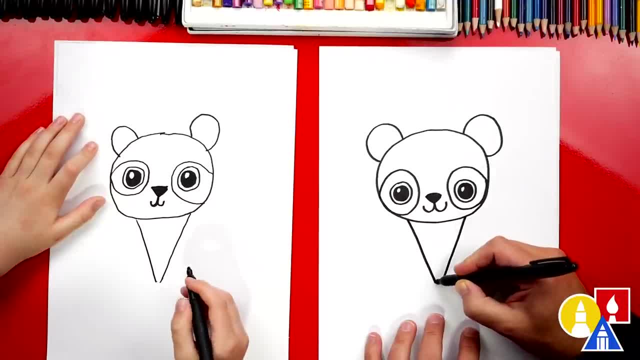 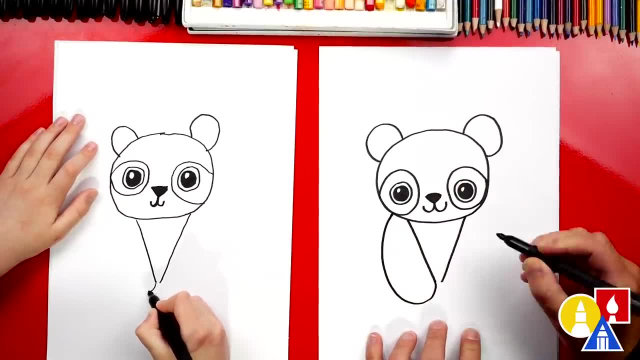 on the right side And we left a little gap down here at the bottom. We're going to curve around and we're going to draw the whole arm coming back up. Ooh, that's a big. I like how strong his paws. 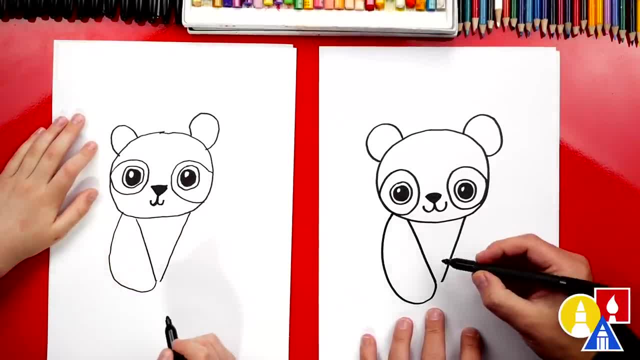 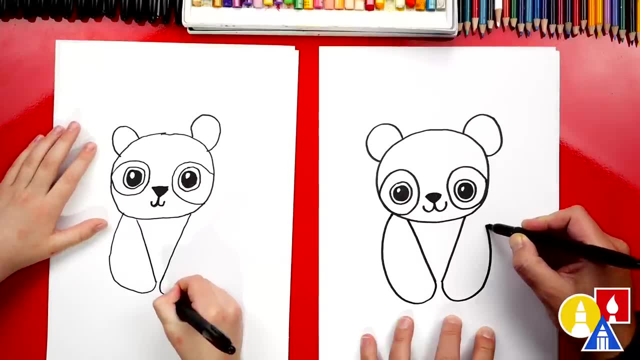 are I like it? Yes, that's perfect. And then let's do the same thing on the other side. We'll curve around. I'm going to try to match the other side. Oh, we did it. I'm going to make the other. 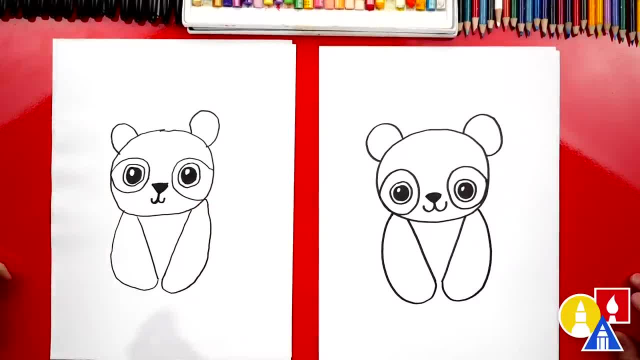 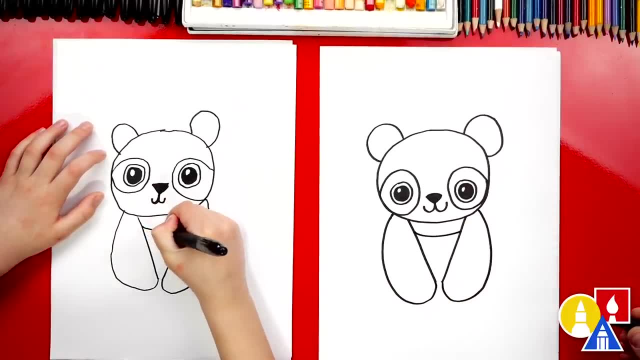 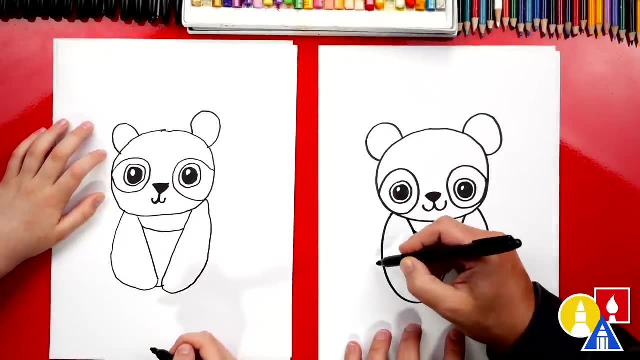 one big because the other one is big. Yeah, you did it All right. now let's also draw a little curve right here underneath the chin, And then we're also going to draw the bottom of the body right here, or his belly, And then let's draw the paws. We're going to draw him sitting down or her. 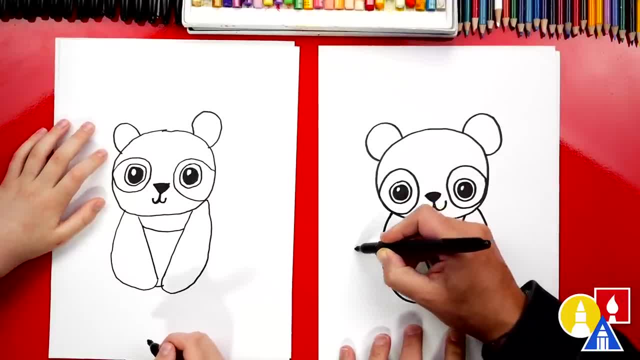 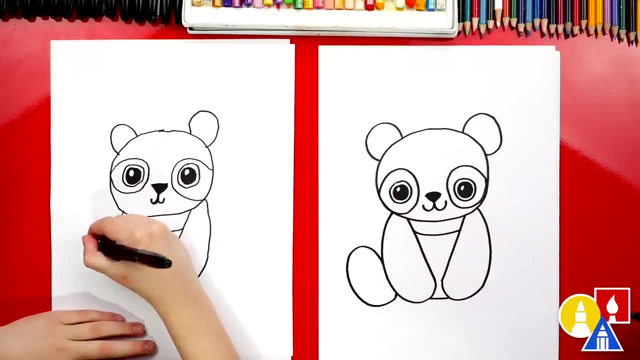 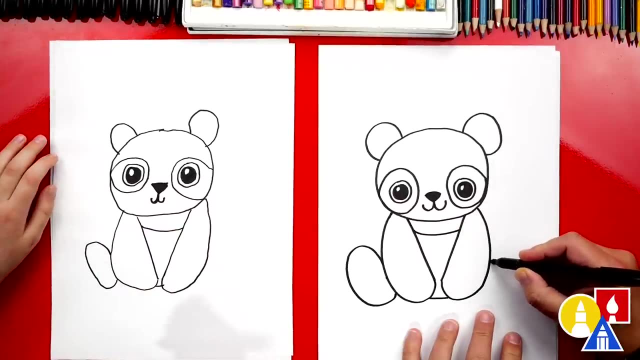 sitting down. We're going to draw an oval shape. We'll come out like this around and then back in. Yeah, yeah, that's perfect. And then let's do the same thing over here on the right side. We'll try to make them the same size. Do you know what it means when it's the same on both sides? 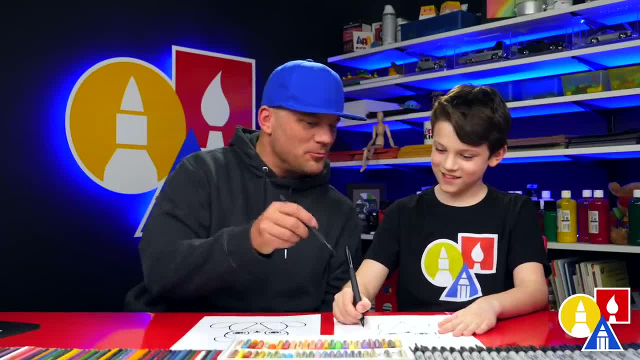 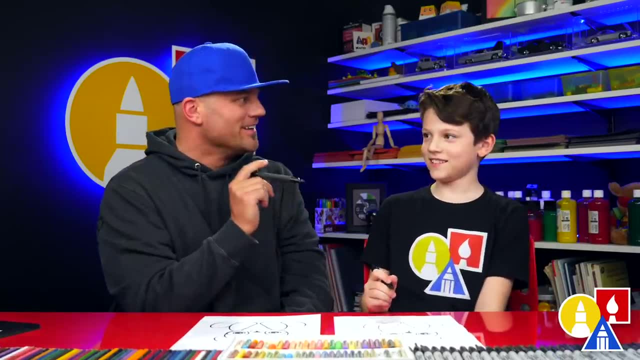 There's a big word. It starts with an S. Oh, keep, keep concentrating on the same thing. I was distracting you and you were looking off into space while you were drawing. That's dangerous. The same situation, Same situation, Symmetry, That's the word. 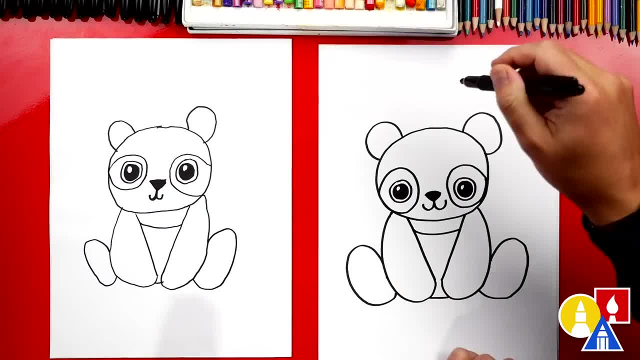 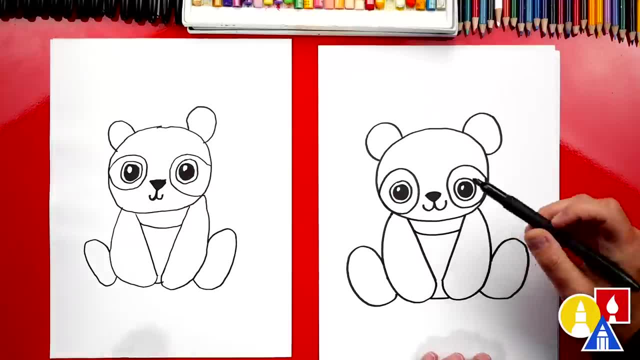 Have you ever heard that before? No, Symmetry means that if you drew a line right down the middle and folded it in half, it's the same on both sides, like a butterfly. Yeah Yeah, If you were looking on both sides of a butterfly, or on our panda bear, it's the same on both sides. 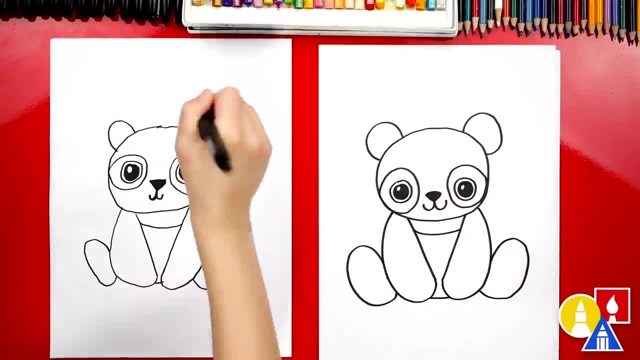 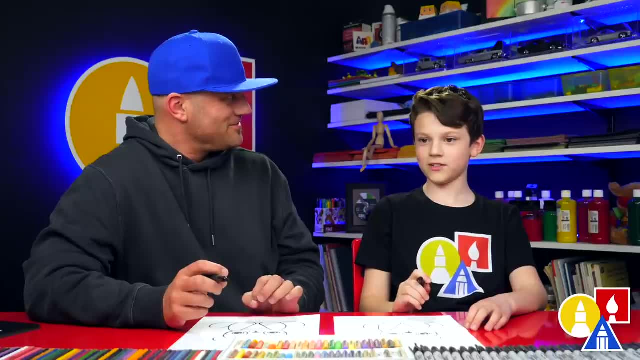 And it has two eyes on the same side, Yeah, And ears- Two ears- on the same side, Yeah, That's called symmetry or symmetrical. Can you remember that? Yes, Symmetrical, Symmetrical. Next let's draw the paws. 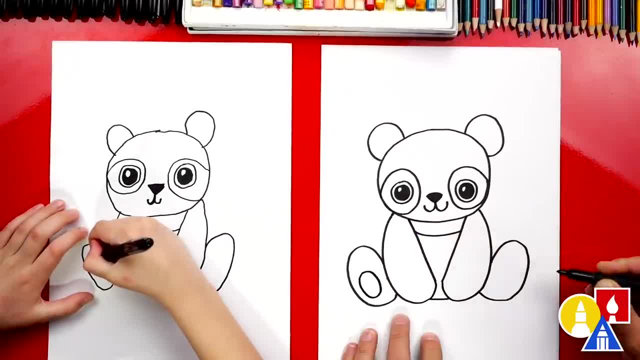 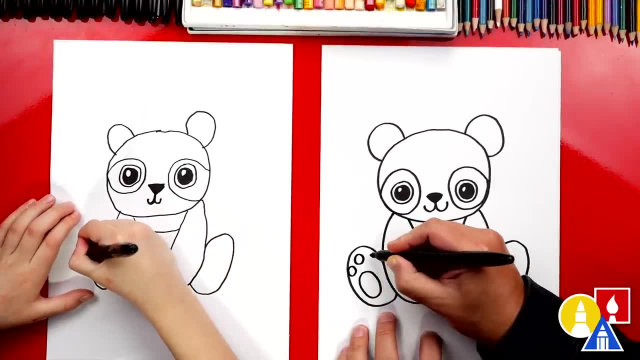 Prints on the bottom of our panda's foot. I'm going to draw a smaller oval down at the bottom, Yeah, And we could draw three circles above it for the toes- Pandas have more toes than that, but we're drawing a cartoon version. 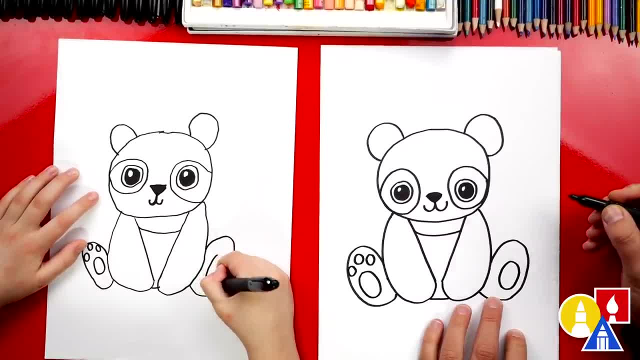 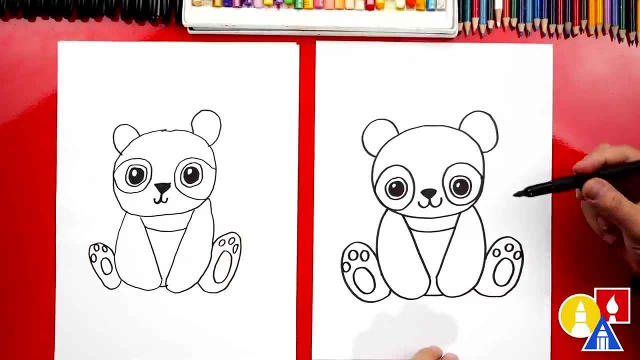 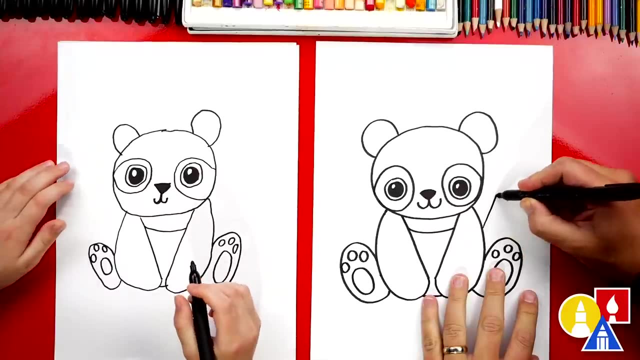 Now let's draw the same thing over here on the right Symmetrical. There you go: Super symmetrical, Super symmetrical, And then three circles for the toes. What do pandas like to eat Bamboo? Yeah, They like to eat bamboo. Let's draw some. We're going to draw a line sticking out right here, We'll draw. 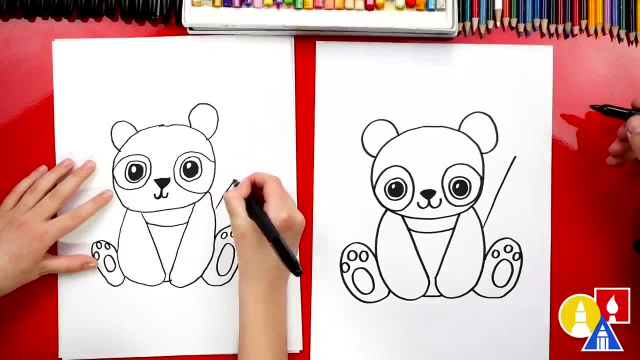 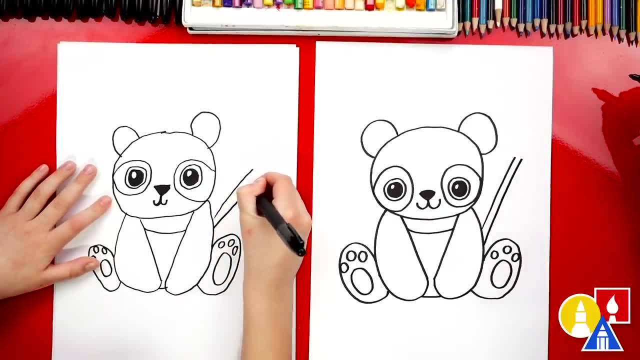 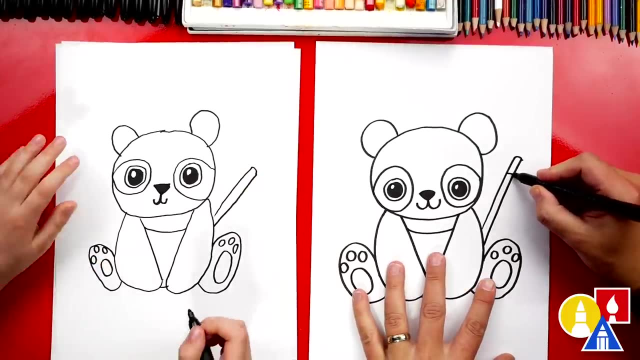 one on the right side. There you go, And then let's draw another one right next to it. This is for the other side of the bamboo stock, And then, up at the top, let's draw a curved line, And then we can also draw curved lines coming down for the rest of the bamboo. It has little segments. 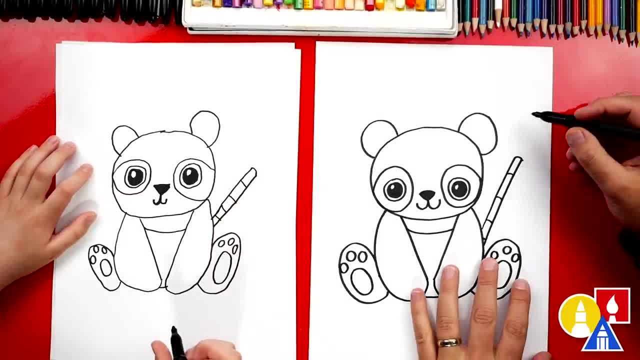 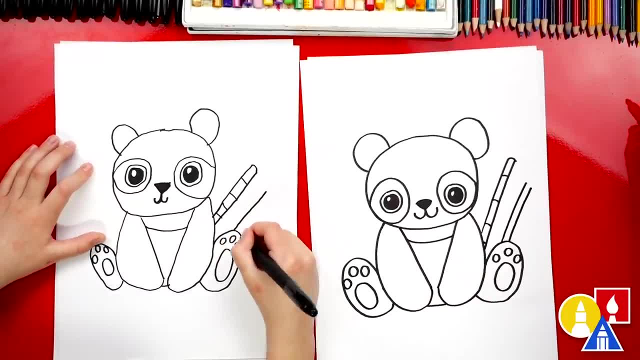 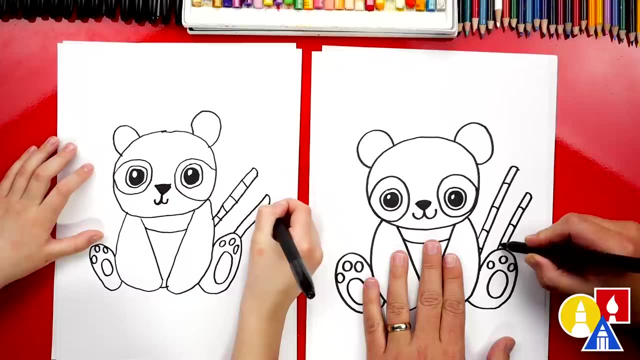 That's what I think makes bamboo really cool. Now let's add another bamboo stock right next to it. We'll draw two more lines- Maybe these ones aren't as tall. There you go, And then we'll connect the top, And then let's draw a couple more curved lines coming down the stock. 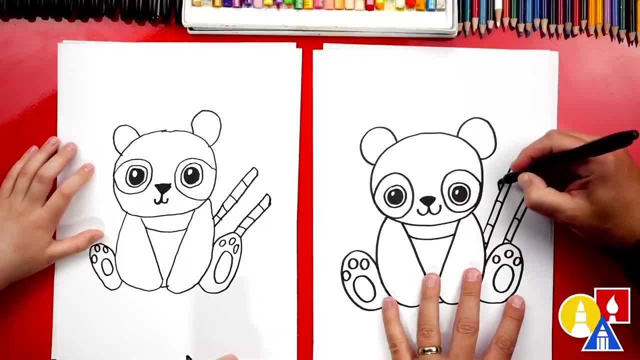 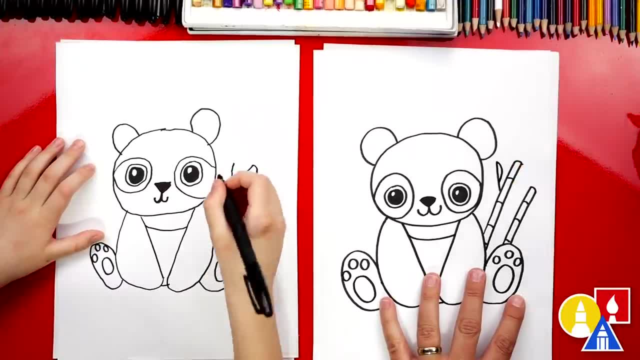 Cool, All right, Let's draw the bamboo leaves. I'm going to draw a diagonal line that comes out And then let's curve Back. There's one leaf. Let's draw another leaf. on the other side, We'll draw a diagonal. 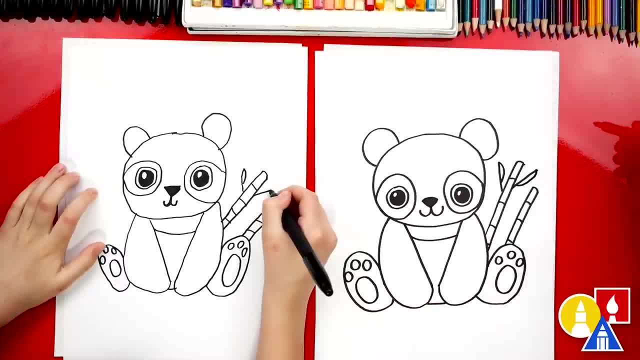 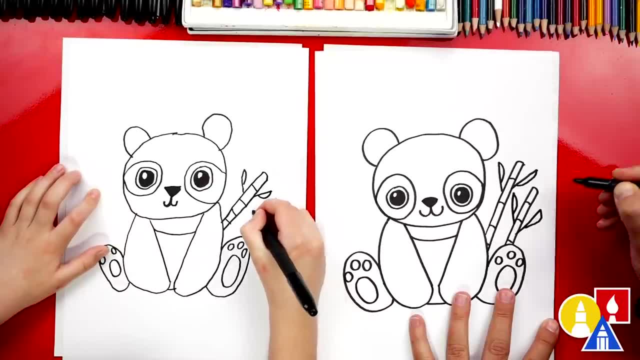 line coming out. Then let's draw another curve coming back for the rest of the leaf. Let's do a couple more leaves. Just repeat that same step over here on the other side. Well, that looks cool. We could even add more leaves, but I think I'll leave it just like that. 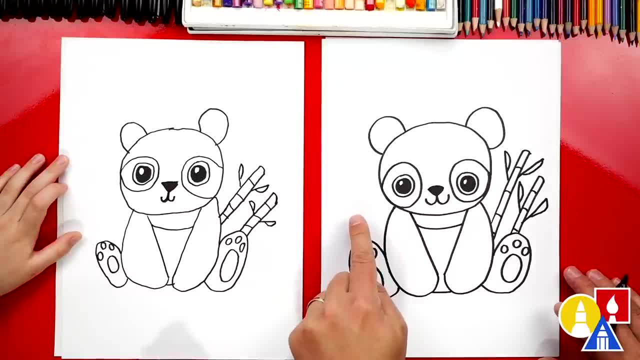 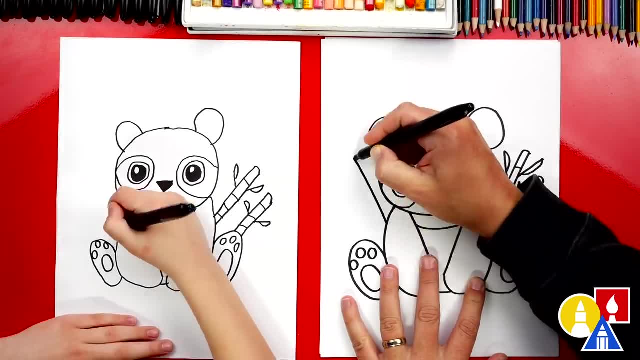 Now we're going to draw more stocks of bamboo over here on the left, but we're going to fast forward this part because we're just repeating the same steps. All right, You ready to fast forward? Yeah, We did it. We finished drawing our panda and also our bamboo. 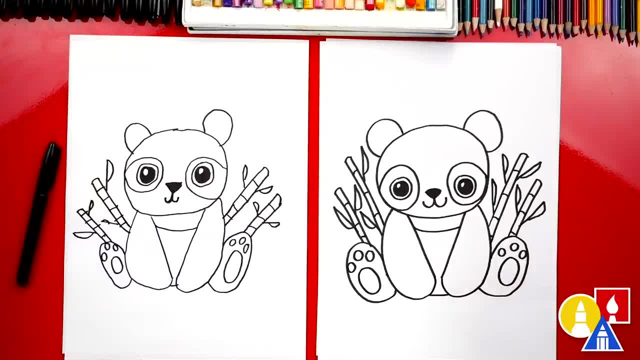 The cool part about that is you could remember those steps pretty easily and add bamboo to a different drawing. What do we still need to do to our drawing Color it? Yeah, this part we're going to fast forward again. At the end you could pause the video if you want to match our same coloring. 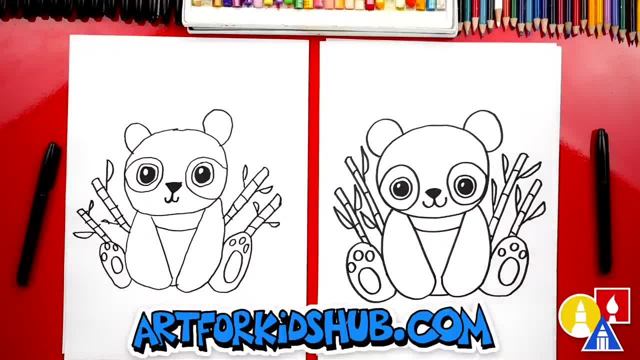 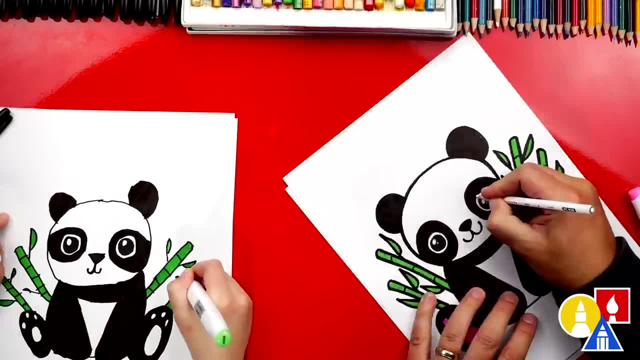 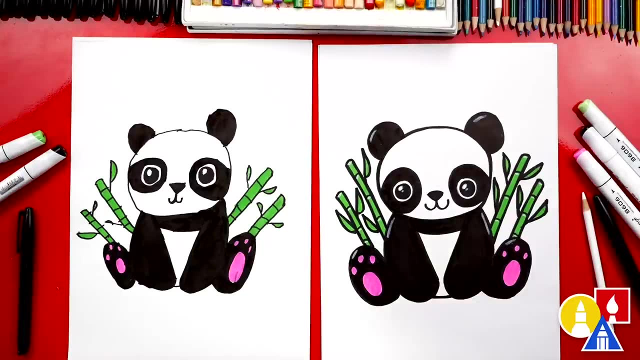 It's going to be pretty easy though. Black and green. Yeah, You ready. Yeah, Awesome, Give it five. You did awesome on coloring your panda. I love it. Do you think it looks better all colored in? I like yours better all colored in? Oh, thank you, I do too. 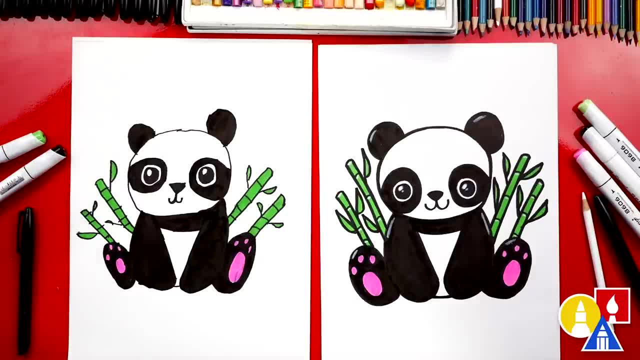 I hope our art friends are going to take time to color their drawings. Also, you could add even more bamboo in the background. That would be awesome. Maybe a whole forest, A whole forest of bamboo and more pandas. That would be really cool Yeah. 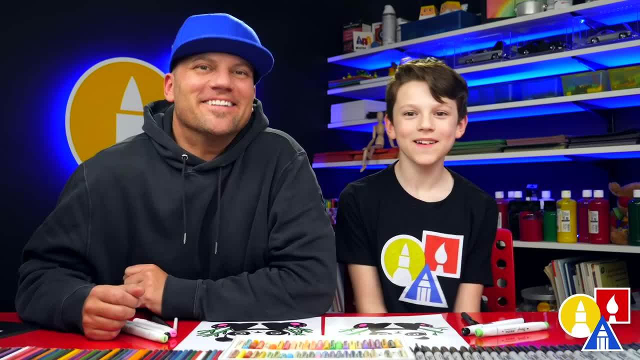 We hope you had a lot of fun drawing your panda. We'll see you next time. Bye-bye, We do. We hope you had a lot of fun and we'll see you later. art friends, Goodbye. 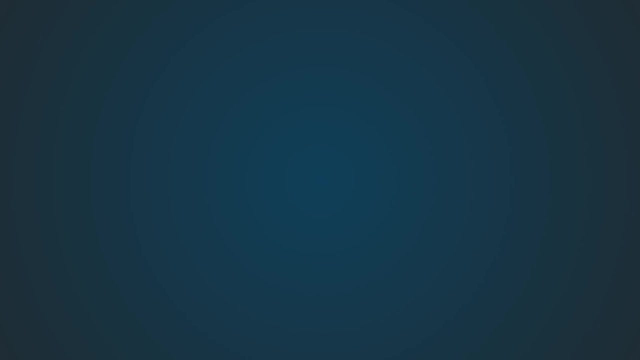 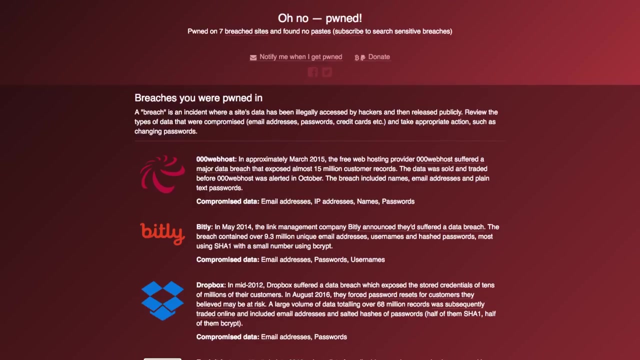 You might have found out that there is a website that checks if your online accounts have been compromised by hackers. So you enter in your email address and, oh no, you have been pwned. Hackers now know the passwords that you used on all these services. 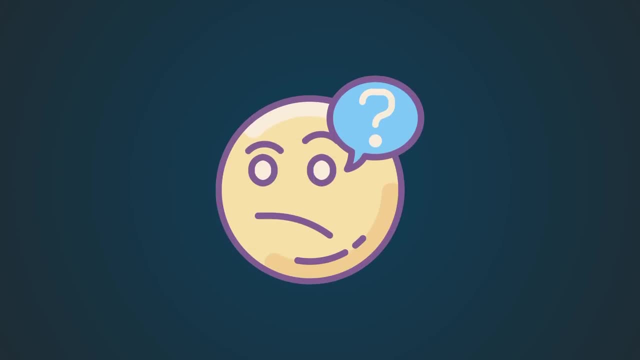 But do they really know your password? Well, as it turns out, that might not actually be the case, And to understand why, let's take a look at what options companies have to protect your passwords and safely store them, so that, even when hackers get access to their systems, your password stays. 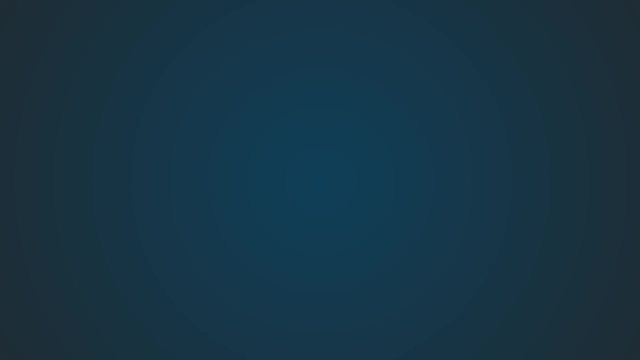 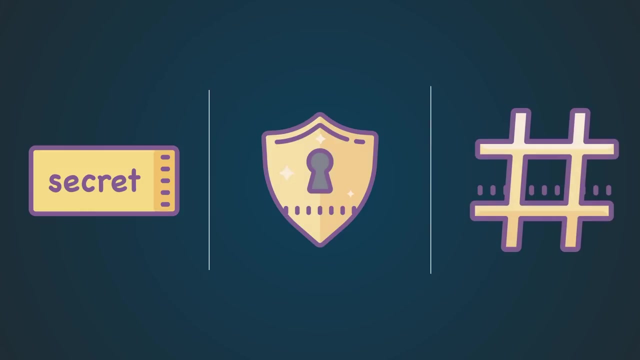 safe. There are three ways a company can store your password. They can store it in plain text, use encryption on it or use what's called a hash function. Let's go quickly over each one of these and let's start with the most basic one. 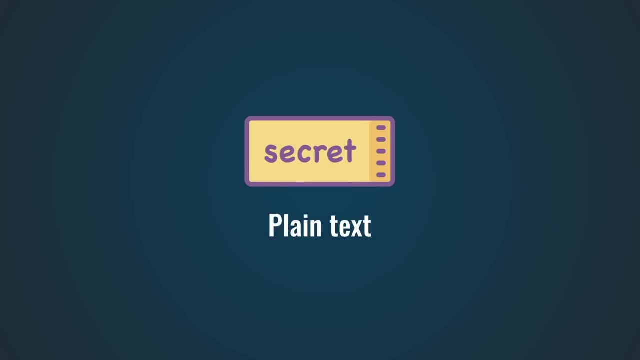 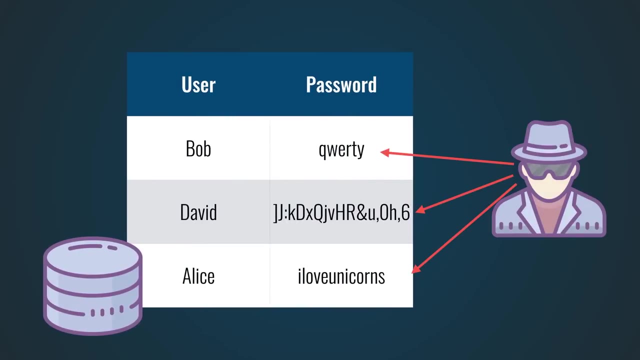 plain text. This is obviously the most dangerous way of storing passwords. If hackers breach the company's database, they get to see all the passwords of the users And since a lot of people have the bad habit of using the same password for multiple accounts, 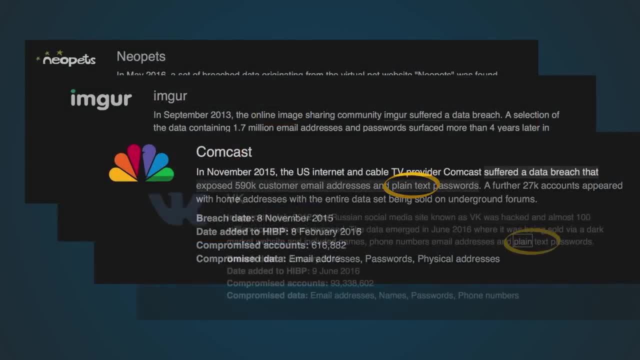 companies with millions of users weren't adequately protecting passwords. A possible alternative to plain text storage is encryption. You take the password you want to store in plain text and use it in plain text. You take the password you want to store in plain text and use it in plain text. You take the password you want to store in plain text. You.